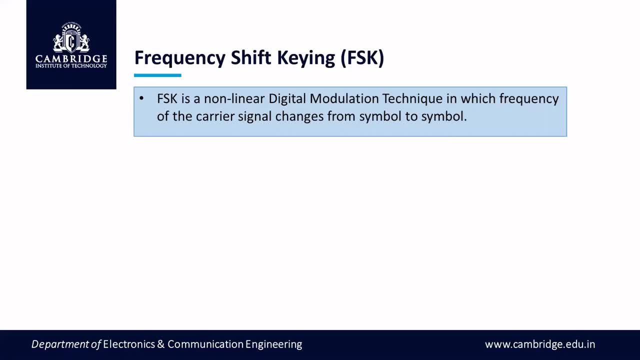 basis function is varied in accordance with changes in input digital signal. The other two characteristics of the carrier signal, that is, amplitude and phase, are kept constant. Since the amplitude of the FSK signal is kept constant, it is not easily affected by the noise. 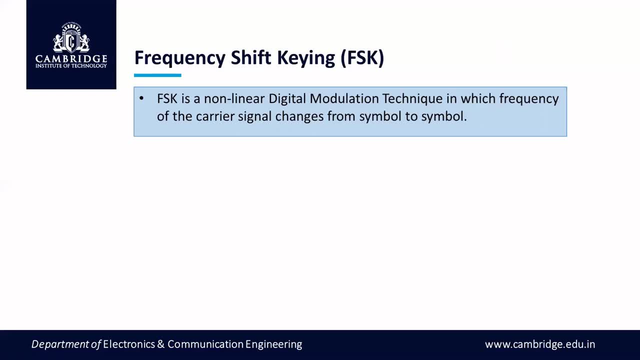 Because the noise is assumed to be additive in nature. when the noise is added to the transmitted signal, So at the receiver we remove the amplitude fluctuations using appropriate circuitry, So because the information is stored in the transmitted signal in the form of frequency variations. 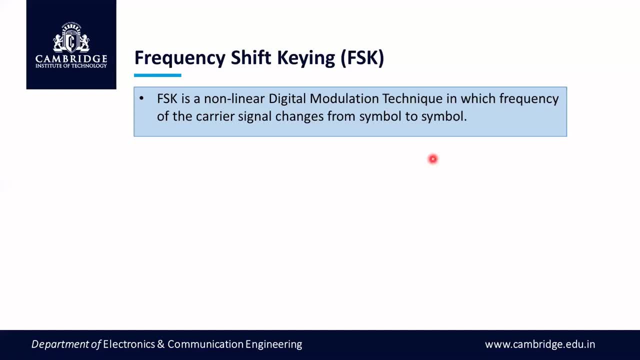 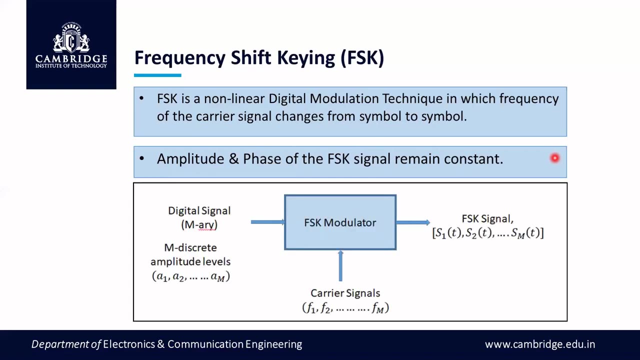 As i said, the amplitude and phase of FSK signal is the same. So, but how do we conduct the queue too? using poor circuit. largest oscillator signal remain constant. Let us look into generalized block term of FSK modulator. It has two inputs. 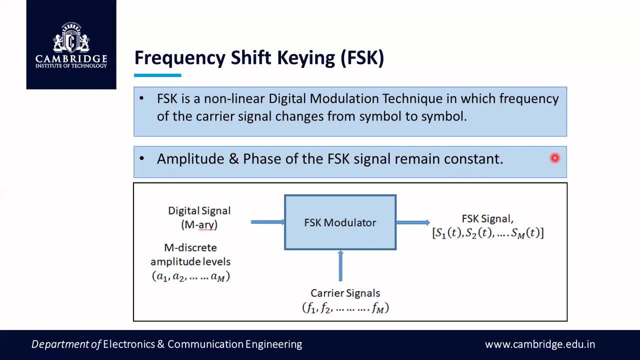 One is the digital signal, other one is carrier signal. In modulation the digital information is transferred to the carrier signal by varying one of its characteristics. But in FSK we vary the frequency content of the carrier signal in accordance with digital signal. 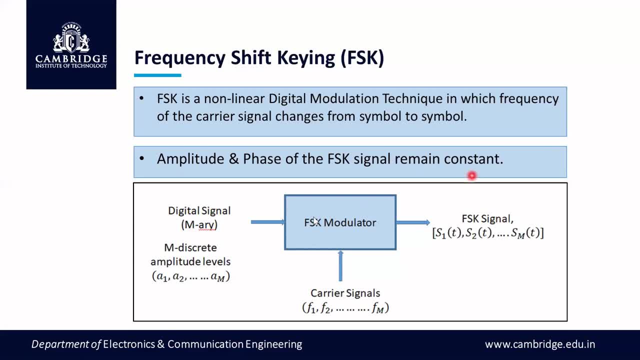 Digital signals are discrete right, So they may contain a fix number of symbols. If the number of symbols in the digital source are m, then the system at higher frequency can is called m array, digital system right and these m array or m number of digital symbols. 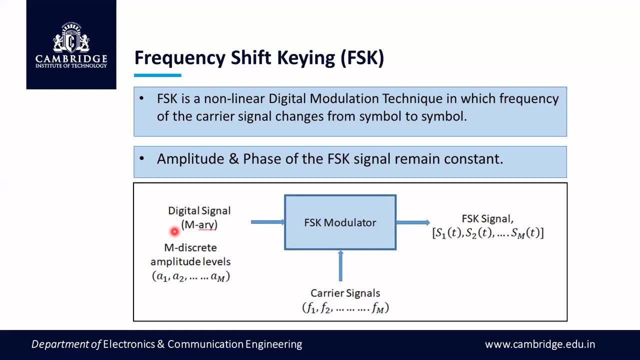 are represented by m discrete amplitude levels. before modulation, these m number of discrete amplitude levels, which i have denoted here as a1, a2 up to am, are transferred to carrier signal in the form of variations in the frequency of the carrier signal. that means the amplitude level a1. 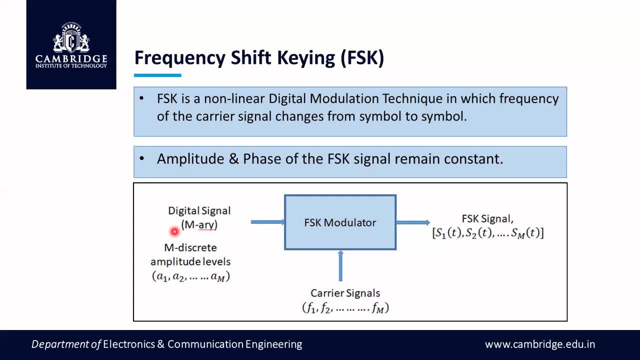 is representing the frequency f1 of the carrier signal. similarly, amplitude a2 is represented by the frequency f2, and so on. so the information, which was in the form of voltage values or amplitude, is converted to the frequency changes in the carrier signal and later they are transmitted on the channel. 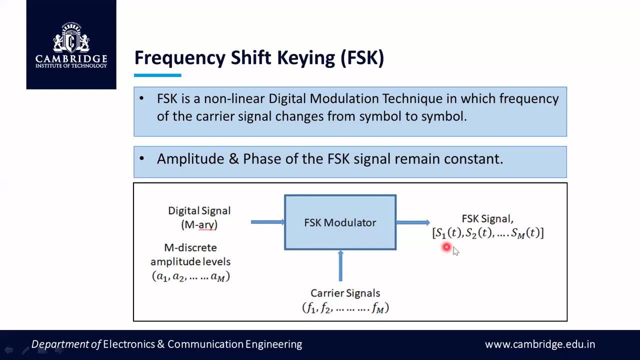 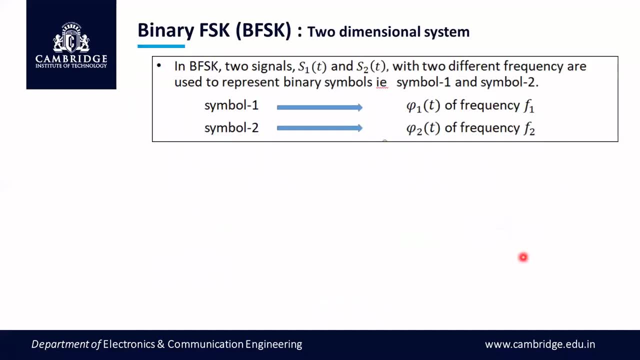 and these signals transmit. signals are denoted as s1 of t, s2 of t and so on. in bfsk the information symbols are two. in mfsk, that is mre, fsk, we find m number of symbols. so bfsk is treated as a special case of mfsk. so only two input symbols. 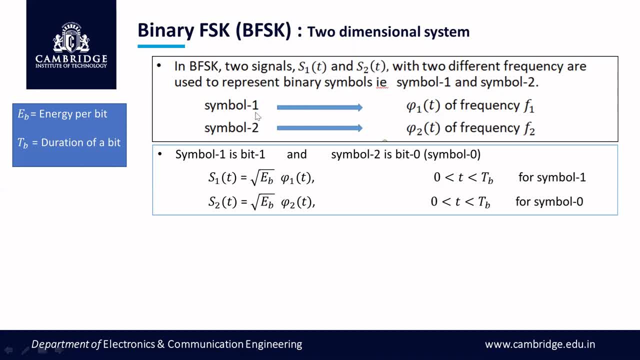 single one emitter. and these two symbols are represented by two different signals, and many of them is a frequency of one and f2, as i said. so accordingly, i am going to define two useful signals for transmission, that is, phi1 of t and phi2 of t. 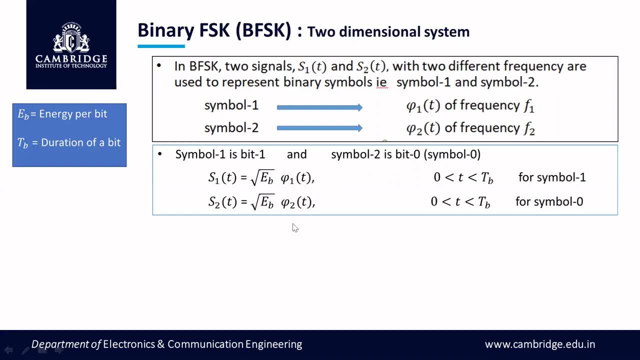 phi1 and phi2 are selected keeping channel characteristics in mind. they are suitable for transmission, overall communication channel. okay, their frequency content, the frequency content of phi1 and EF2, 16-1 of t are small and totaliles within an array. Here we have three signals, 5 and two simple signals. they will carry externaligung over these signals, over a wave passengers, over a wavegeb centralized to theصg, to theondo-gegon, etc. output of 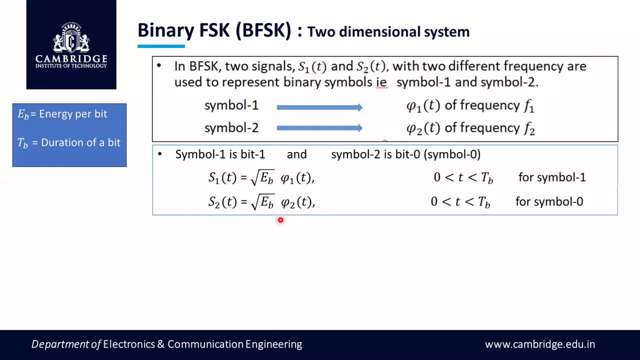 of phi1 and phi2 are containing information, Hence their aptitudes remain same. Rho dv will remain same for both the symbols. Now I come to the mathematical definition of the BFSK signal, That is. the FSK signal is denoted as S of t. 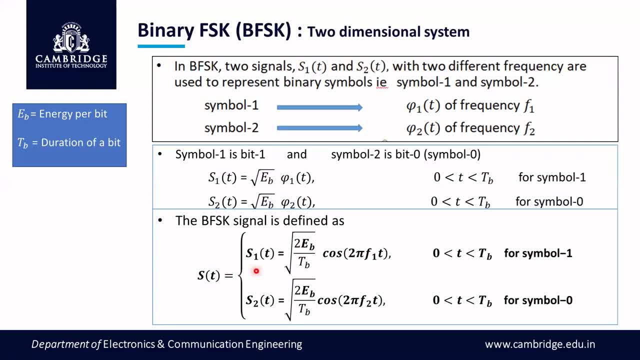 S of t, which can be either S1 of t or S2 of t, depending upon the symbol generated by the source, Symbol 1 and symbol 0.. For symbol 1, the signal, what I had told, that I have selected carefully: phi1 of t. 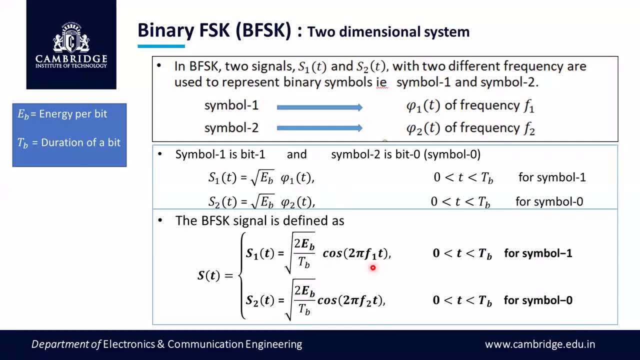 is now going to be sinusoidal signal: cos2, pi, f1 t. Similarly, for another symbol, it is going to be cos2 pi, f2 t. f1 and f2 are different frequency signals, So f1 and f2 are different. 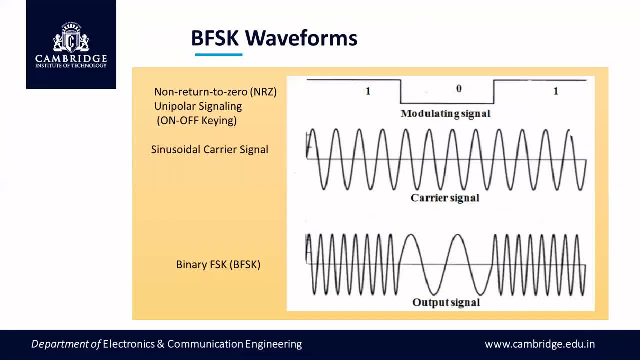 values. Let us look into the waveforms of binary FSK. As I said, we have here the input signal, which is called binary signal. This binary signal is having two discrete amplitudes, As I said in the beginning, in M-ary system. 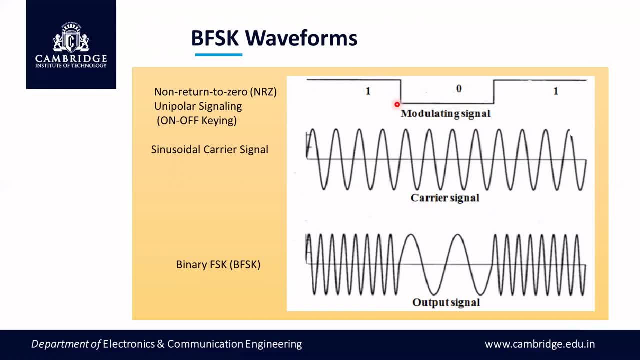 M number of discrete amplitude levels are used, But in binary only two amplitude levels are used. Let us assume one value is plus one volts, other value is zero. So I am going for positive value and zero value, which is similar to our. 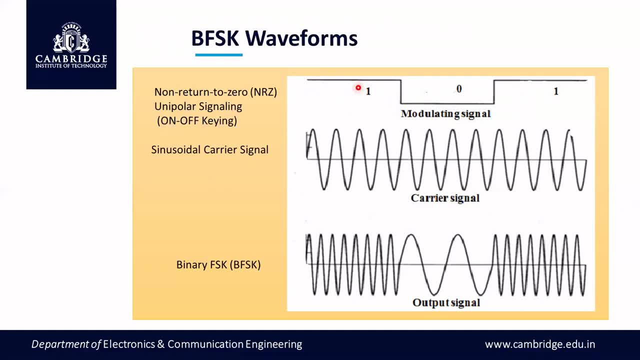 ANOV keying technique, that is, unipolar signaling. The input binary sequence is represented by this strain of rectangular pulses having positive pulse and zero amplitude pulse. We use this one and zero values for amplitude because just by multiplying the signal with this sinusoidal carrier, 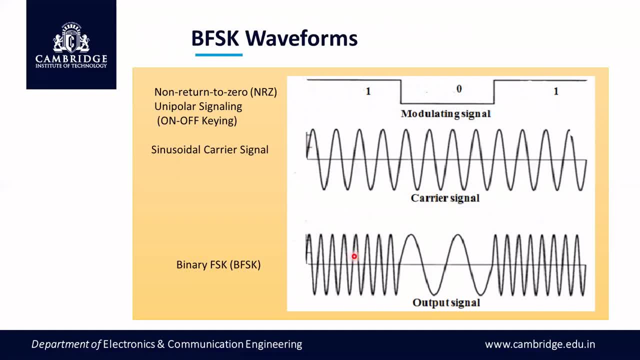 we try to get FSK But it is not possible. But with little bit modification we can do. What is that? one is: When you multiply these two, then one amplitude is multiplied with carrier signal. carrier signal remains same Here: one amplitude multiplied with carrier. 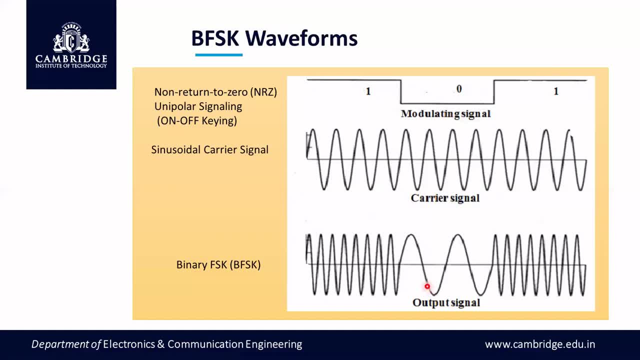 carrier remains same, But this fellow is converted to zero. So this signal that is representing bit zero is of different frequency. So we need to have two carrier signals. Here only one carrier signal is shown, just for an example. Similarly, there is going to be one more. 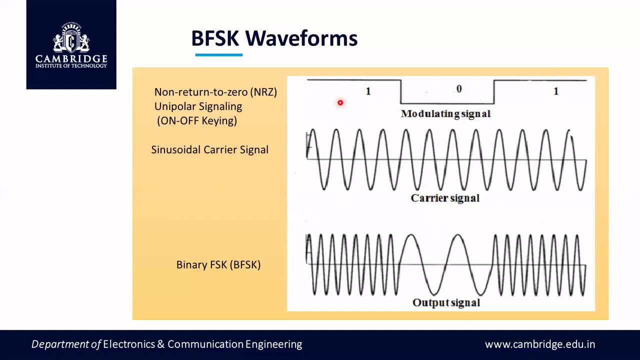 carrier signal of different frequency, of this frequency So that we should plan later in the transmitter that one should multiply carrier one, zero should multiply carrier two, so that we get this waveform Right. One important information to be known at this point of time. 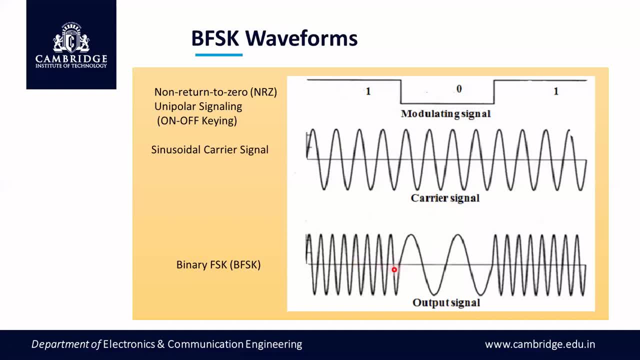 is: look at this, Even the frequency is changing, but at this point the signal looks like continuous. Here also the signal looks like continuous. Frequency is discreetly changing, but the phase value, that is, delay value, is continuous. 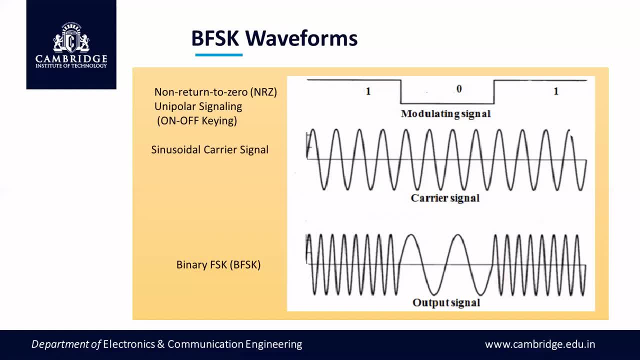 So FSK is a non-linear modulation technique in which frequency abruptly changes from symbol to symbol or discreetly changes, but the phase of the FSK. phase of the FSK varies linearly. So there is no discontinuity in the signal. There is no discontinuity. 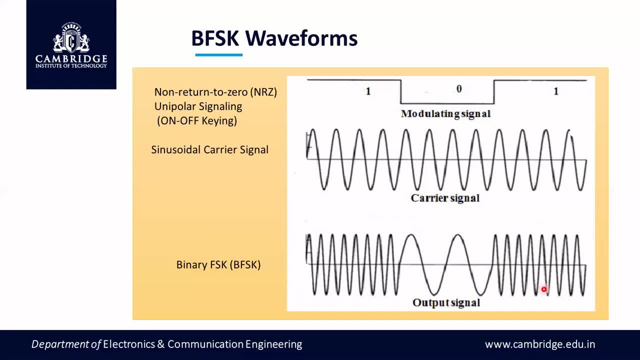 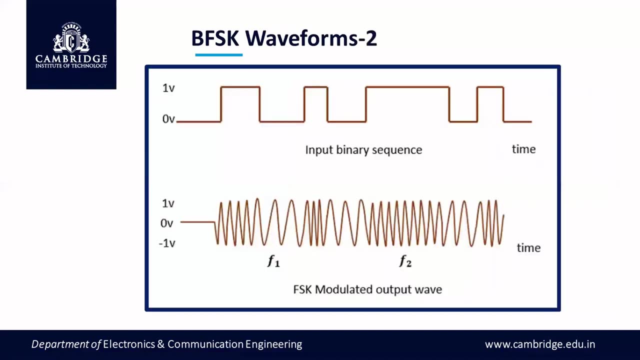 in signal goes continuously till the end. So this makes the delay a linearly varying quantity. That means linear phase. The linear phase of the FSK signal is appreciable quantity for many reasons. So we have given one more waveform for better understanding. 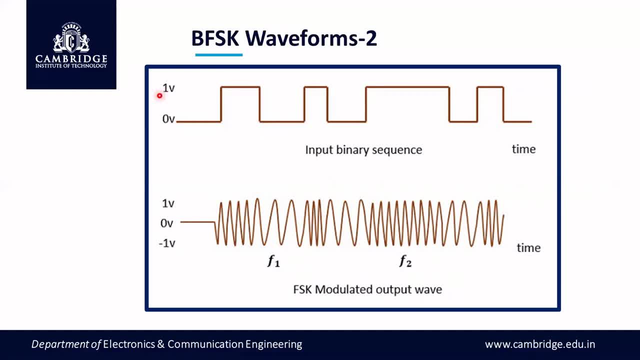 Look at this: As I said, I have chosen one volt for positive pulse, zero volt for another pulse. So these one and zeros represent the frequency, And here is the final FSK signal. See: positive pulse, one frequency, Zero pulse. 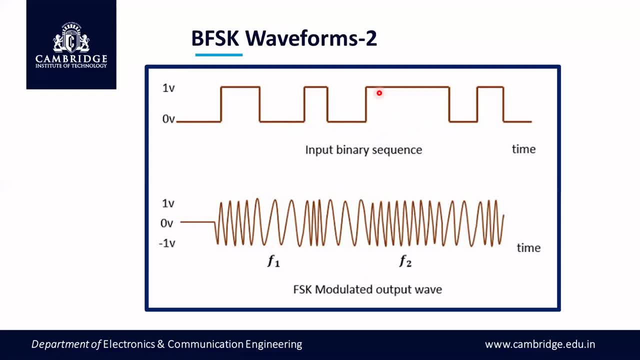 different frequency. Positive pulse, same frequency. Here it is duration Z. This duration is two times this duration. That is why there is going to be two bit ones And this is one zero one. So looking at this, we can easily 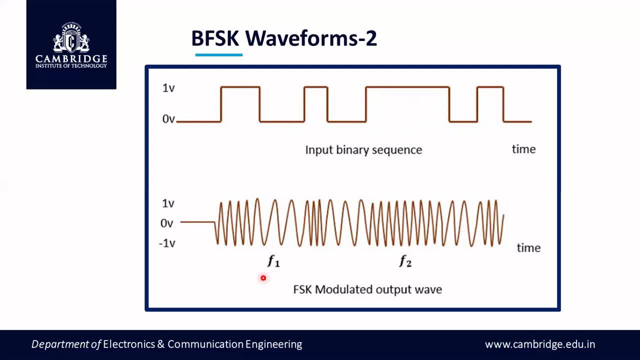 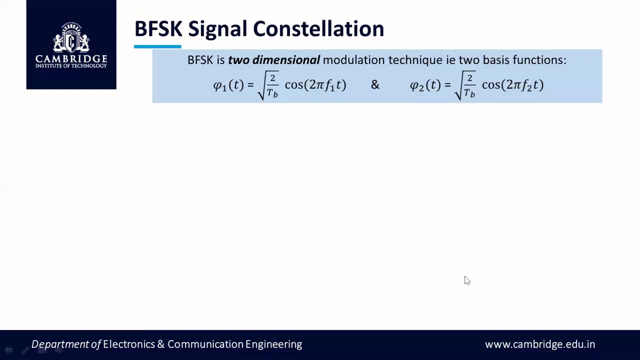 understand how to write an FSK waveform. Here it is denoted as this frequency is taken as F1 and this one is taken as F2.. So we can easily understand how to write an FSK waveform. Let us look into the mathematical interpretation of. 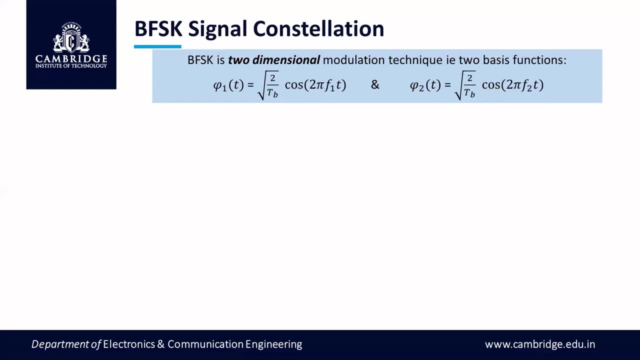 FSK signal, Since we are using here two different frequencies. two different frequencies to represent two different binary symbols. So we need two carriers, nothing but two basis functions. So FSK is two dimensional modulation technique. The basis functions, what I was talking, are: 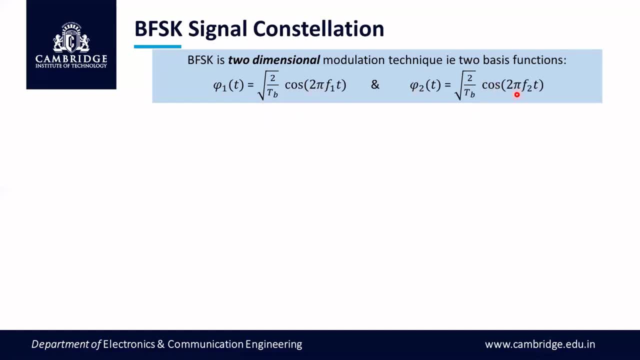 phi1 and phi2.. So they are basically sinusoidal signals, Signals of frequency of F1 and F2.. Their amplitude remains same. So we know that root of 2 by dB is chosen to make this energy, of this basis function. 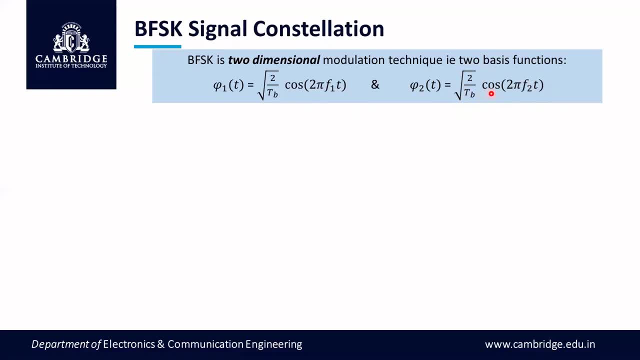 unity. If we calculate the energy of this basis function with this amplitude, we will get one. So, keeping that in mind, this amplitude is closed up. Now the equation for VFSK is given once again here: S1 of T. 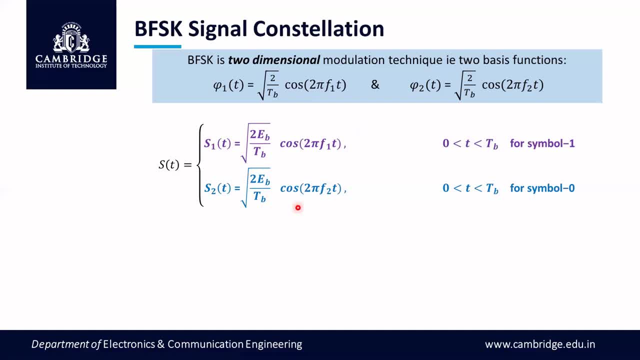 representing one symbol with frequency F1 and this one is with frequency F2.. So now let us introduce the symbols of phi1 and phi2 back into these equations of S of T. So here Eb represent energy in one bit, Tv is the duration of one bit. 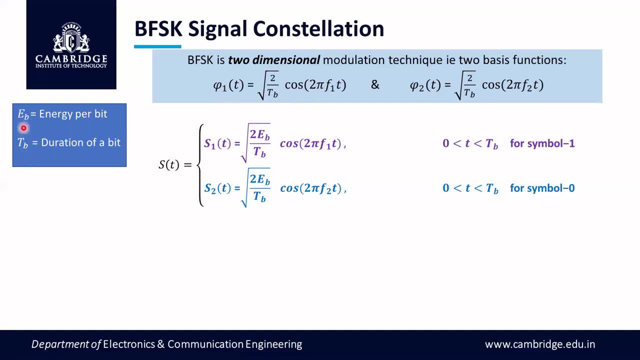 Ok, This energy in one bit duration can be obtained by multiplying this Tv with the power P. So power into time is going to be energy. So energy is calculated by multiplying Tv with the power content of the particular symbol. So in this equation, 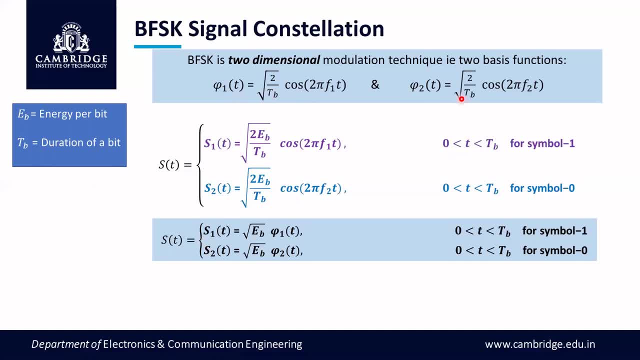 we have introduced these two equations. Ok, The root of 2 by Tv, cos 2, P of 100 A is written as phi1 of T, phi2 of T. So we can say that the amplitudes are same, but the signals. 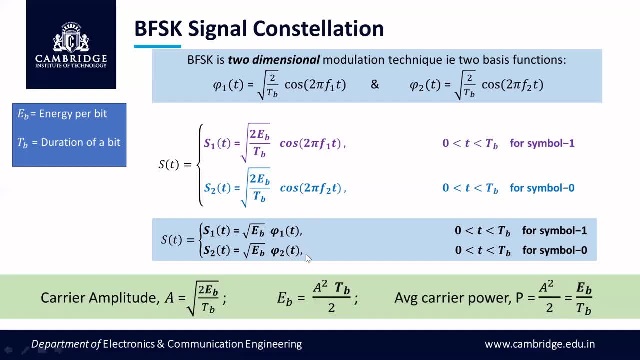 are different in frequency. So before we continue, I would like to stress upon one more point which is useful in solving numericals, This particular thing. Let me use annotations here And look at this one. This value is the amplitude of s1 of T. Similarly, 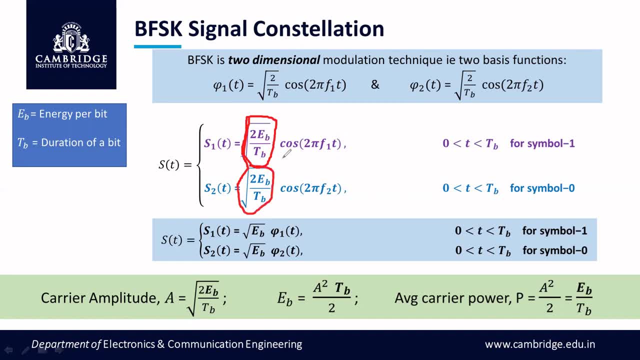 this one is the amplitude of s2 of T. Both of them are same, So the amplitude of the carrier signal here is taken as the same value, Root of 2 Eb by Tv. Ok, So in general in this case we can write it as: 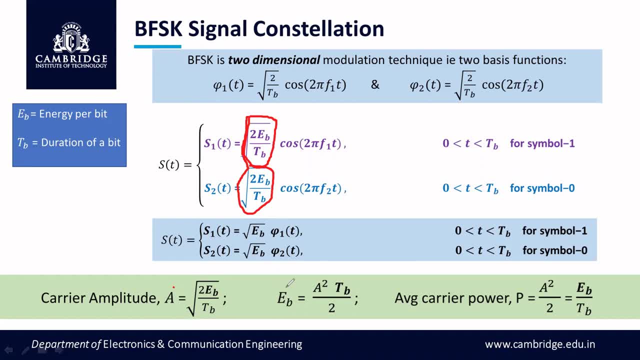 A Right. So now from this equation we can find bit energy, That is Eb. So cross multiplication gives you this equation. Right Now I am going to find average carrier power. This is very much required for us. 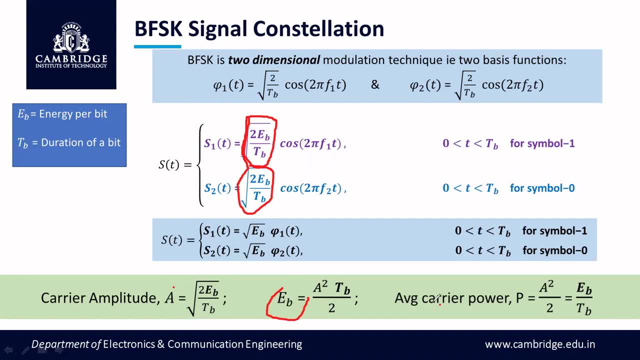 Average carrier power. And we know that average carrier power Power is obtained generally by squaring the signal Right, But here the signal contains a sinusoidal quantity. That is why amplitude is this value. So this value divided by root, 2. 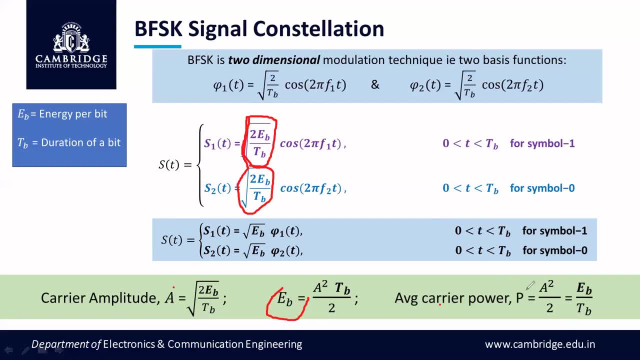 will give you RMS value. Upon squaring we will get power. So it is going to be A square by 2.. A by root 2 is RMS value of the signal And squaring that only to A square by 2.. 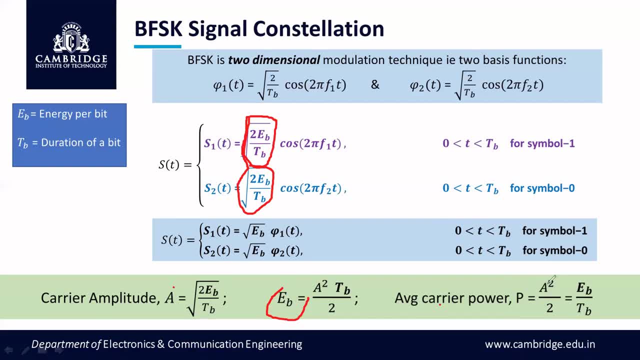 That is the average value, Average power value. So this A square by 2 here, This is the A square by 2.. This A square by 2 is taken over here. So then, from here, if you leave A square by 2, 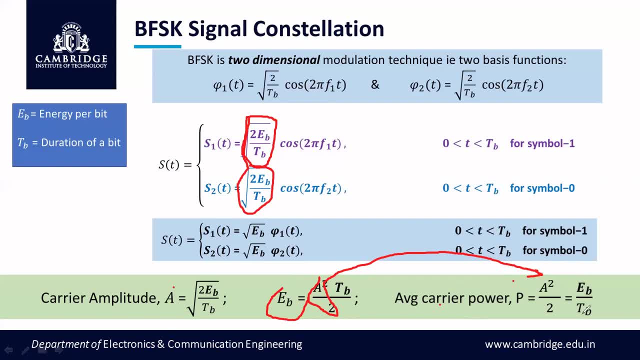 you will end up with Eb by T. So A square by 2 is also equal to Eb by T. Right, A square by 2 is also equal to Eb by T. So keep it in mind that average carrier power is given by. 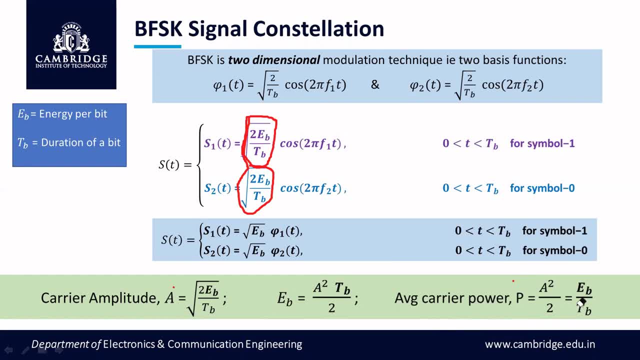 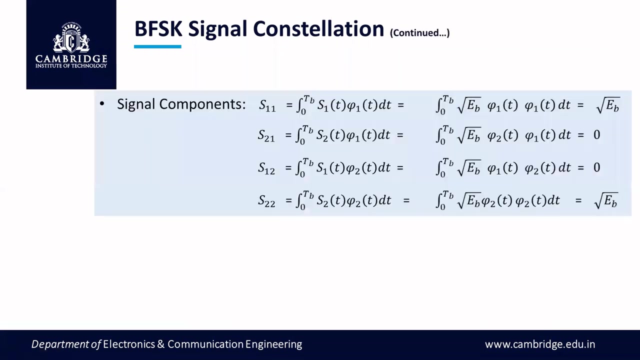 A square by 2 or Eb by T. That is the ratio of energy by time. Energy by time is always equal to the power, Right? So here we know that there are two basis functions. Okay, There are two basis functions. 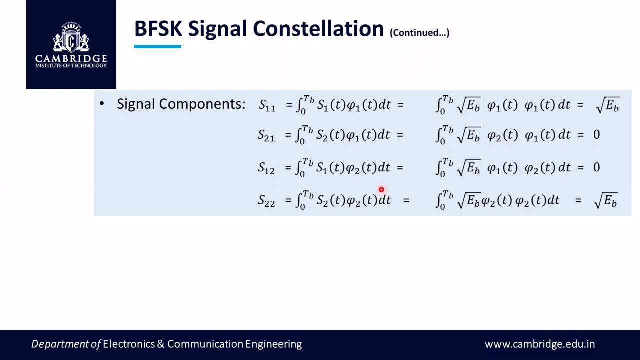 5 and aft and 5.. 5 and aft and 5.. 5 and aft and 5.. And these two basis functions are two carriers carrying the information. These two basis functions are chosen to represent two binary information. Accordingly, we get two signals. 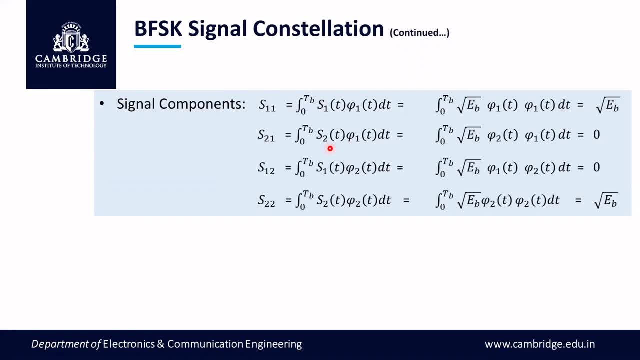 One is S1 of T and another one is S2 of T. Okay, So there are two signals of Fsk, S1 of T and S2 of T, in which either 5 and aft is used, or 5 and aft is used. 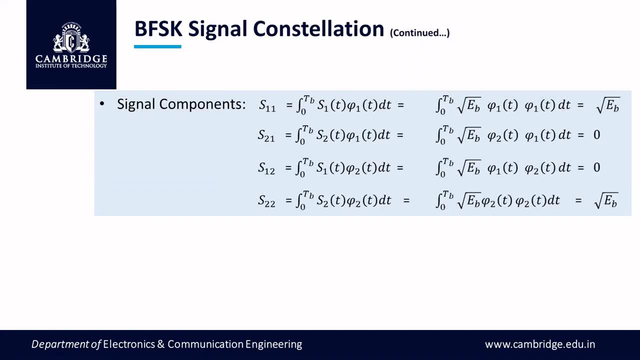 That means the basis functions can be used to represent any of the information symbols. So now I would like to find out which signal contains which basis function. Okay, So what we can do that time is write. we can do this If S1 of T is containing: 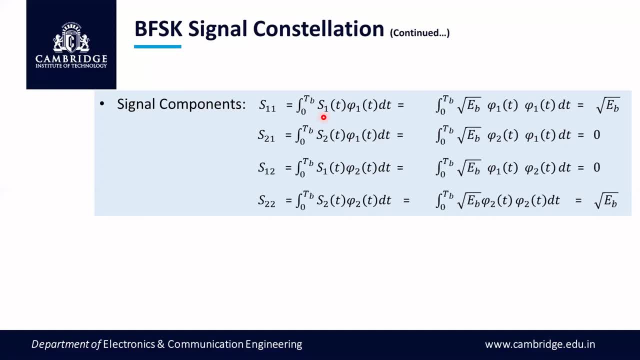 5 and aft, then what happens? If S1 of T is containing 5 and aft, then what happens? Let us take into this. Let us multiply S1 of T with 5 and aft and integrate over one bit duration. 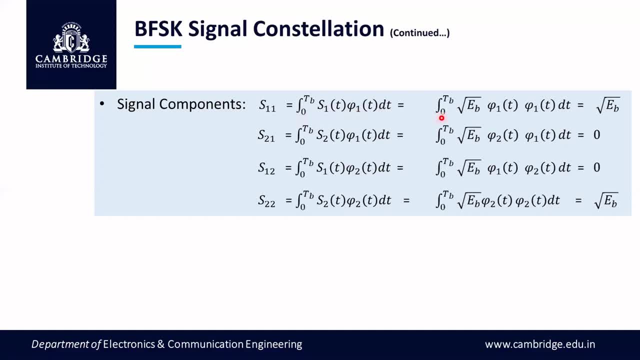 Right. So that time we get this equation In place of S1 of T, I am going to substitute root Ev, 5 and aft. This is what the definition we made in the previous slide. So S1 of T is assumed to contain 5 and aft. 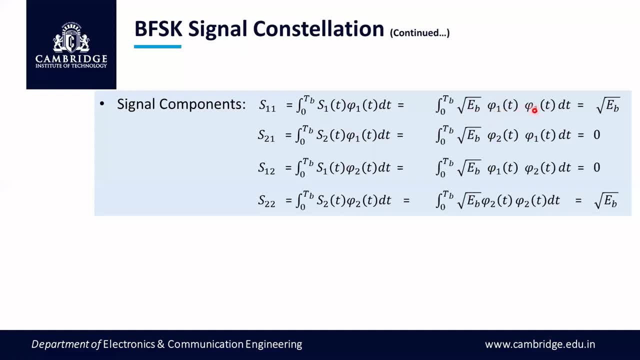 with amplitude of root Ev, So 5, and aft into 5 and aft, So 5 and aft into 5 and aft 5 and aft square, we will get and we integrate this one Root Ev is a constant, So keep the root Ev outside. 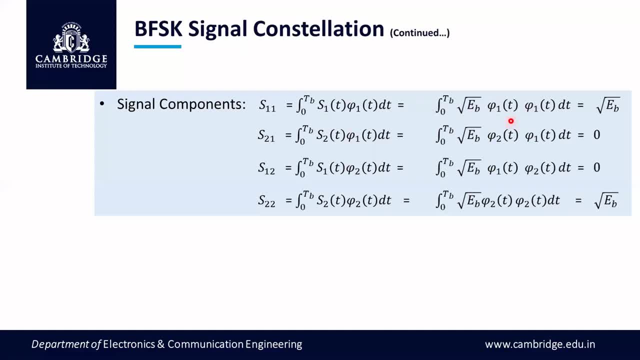 So integration of 5 and aft is always one, because 5 and aft is a basis function. All basis functions are assumed to be orthonormal. That means they are orthogonal as well as normalized, Since they are orthogonal whenever they are multiplied with itself. 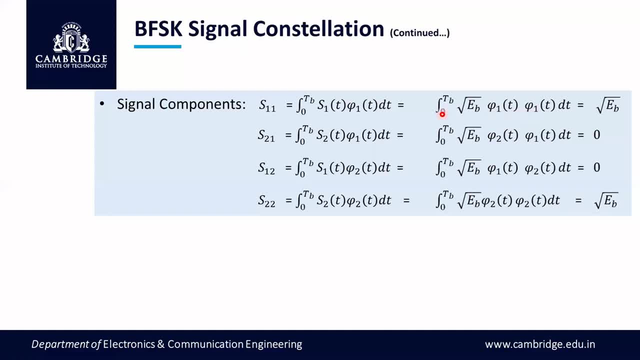 and then squared and integrated, we will always get number one. So unit energy, Because their energy is always one. One into root Ev is root Ev. That means S1 of T contains 5 and aft. Similarly, let us do the discussion with S2 of T. 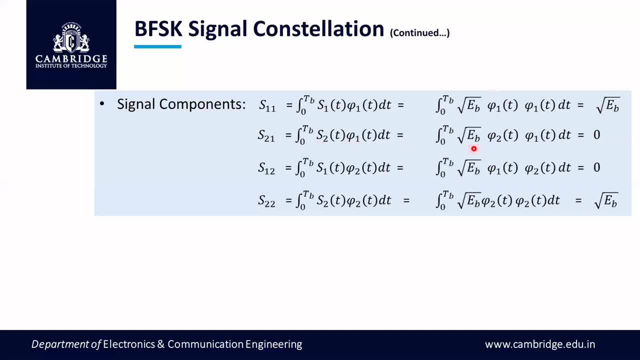 When S2 of T is multiplied with 5 and aft. So definition of S2 of T is root, Ev is 5 and aft, But we are checking for 5 and aft, So 5 and aft into 5 and aft. 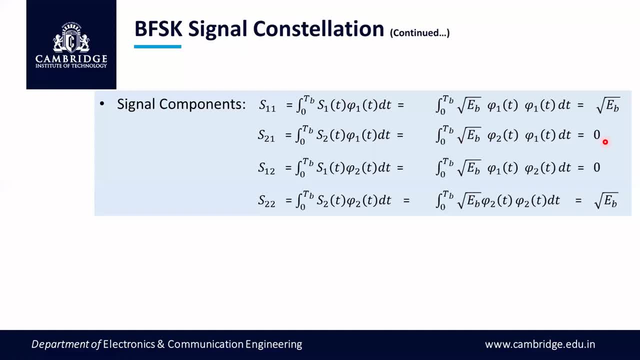 integration always gives zero, because both the basis functions are orthogonal to each other, perpendicular to each other, Nothing. but they have a phase shift of 90 degree. That means they are independent of each other. That is why, when two different basis functions or orthogonal signals are multiplied, 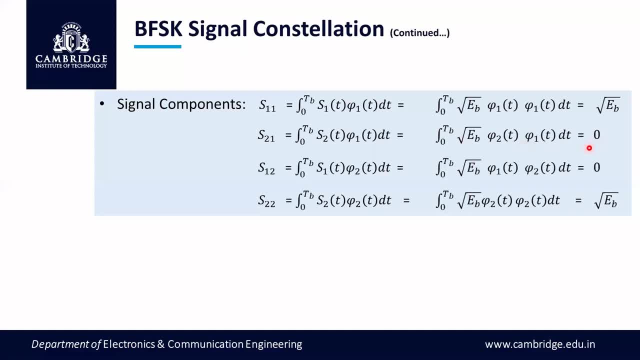 and integrated over a period, we will always get zero. That is the probability of orthogonality. So we come to the conclusion that S1 contains 5 and aft. That is first basis function. But S2 does not contains 5 and aft, That is. 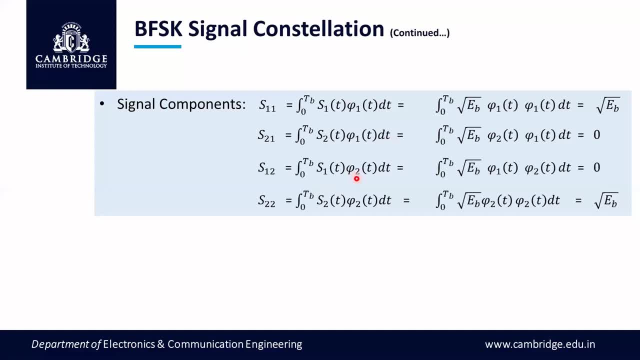 going to give zero. Similarly, when you do with other basis functions- 5 and aft. In S1 of T we do not have 5 and aft. So in S2 of T we have 5 and aft. That is why we get the value root Ev. 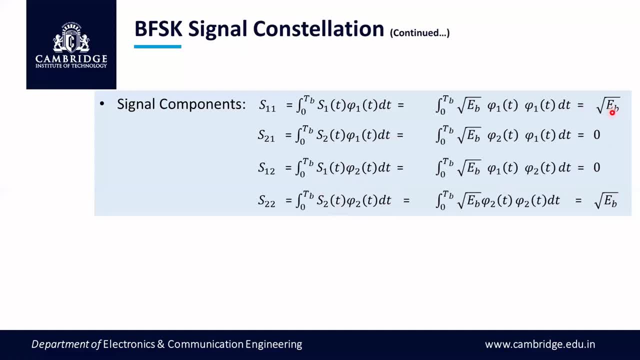 So root Ev. This first root Ev is the signal component of S1 of T. The second root Ev is the signal component of S2 of T. So both S1 of T and S2 of T are having same signal components: root Ev and root Ev. 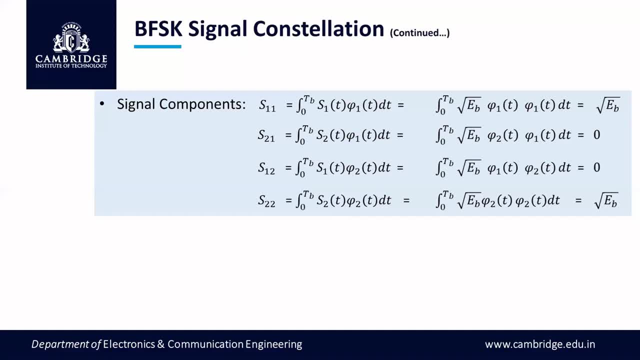 But they are having different basis functions. They do not have this one. So that is why, at the receiver, to identify the symbol transmitted, we always look into this aspect. We do the same thing with the receiver signal. So we multiply the receiver signal once with 5 and aft. 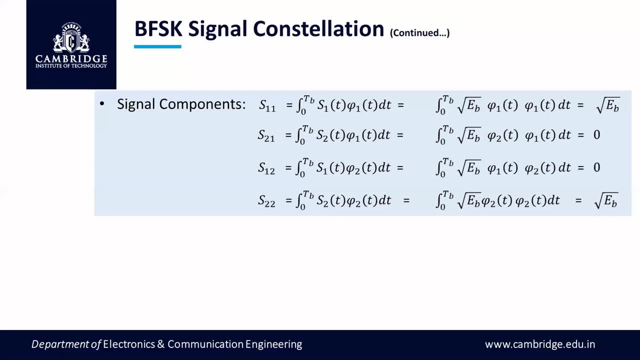 and another time with 5 and aft and we integrate it That time. any one of these two, that is, 5 and aft or 5 and aft, will produce large amount of output. So whichever produce large amount of output, that basis function is of our interest. 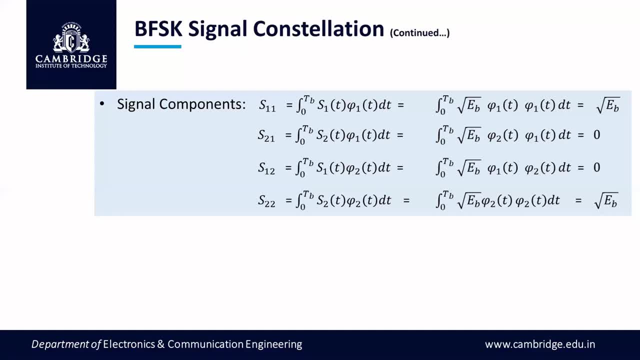 Suppose, when you multiply receiver signal with 5 and aft, if you get more power, that is, symbol 1 is transmitted. When you multiply with 5 and aft, if you get more power or more energy, the symbol sent was 0. So this aspect 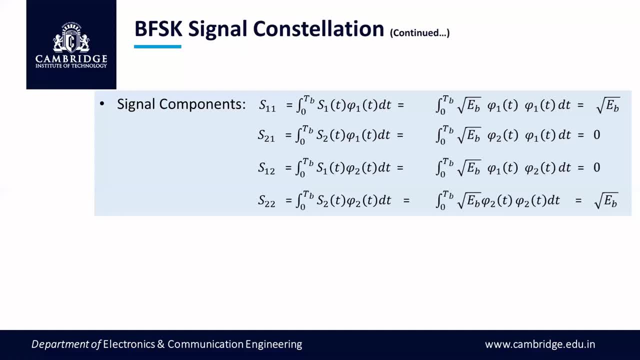 is to be kept in mind. So accordingly, based on these outputs, I made signal vectors. For the first signal, first basis component is root Ev. second basis component is 0.. Here for the second signal, first component is 0. That is first basis component. 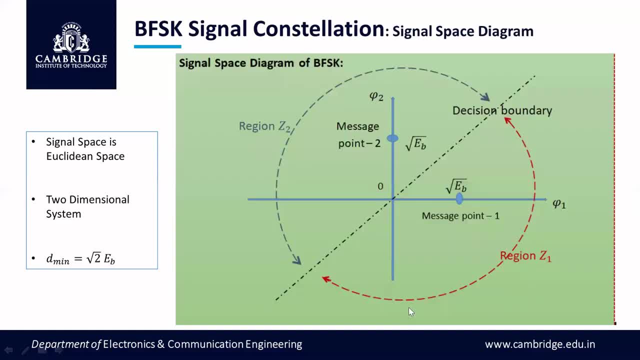 First basis component. Second basis component is root Ev. Yes, Now we will come to the signal space diagram. Let us transfer the signal components into Euclidean space, which is called by name, signal space. In the signal space, every point represents one signal. 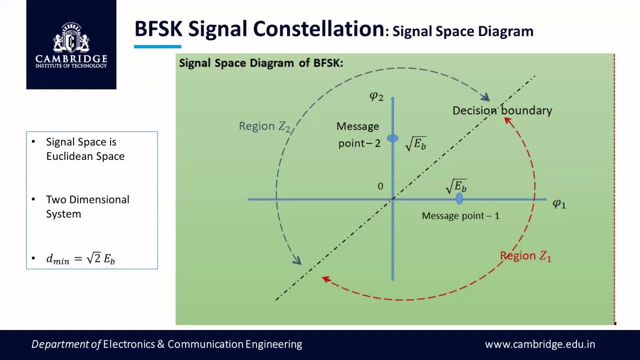 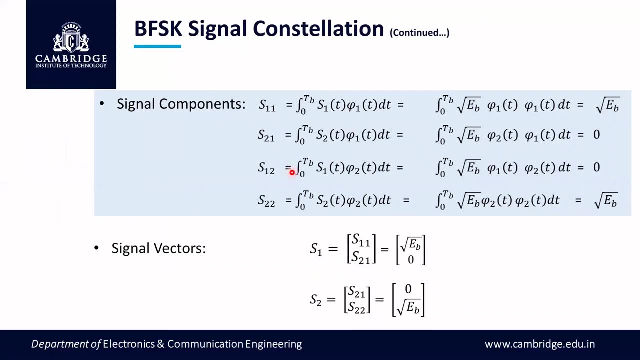 Right, Since we have two different signals in FSK. so we are going to identify two message points in the Euclidean space which represent our signals. Okay, So let us go to previous one and see The first signal. Right, The first signal is having. 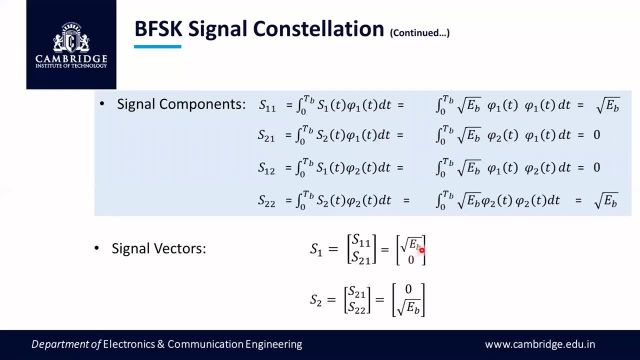 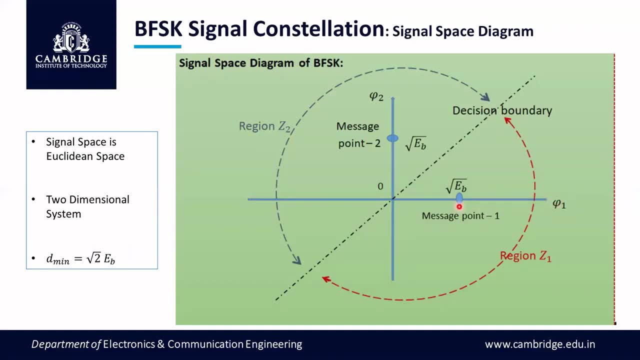 coordinates of root Ev and 0.. Root Ev is 5-1 component, 0 is 5-2 component. So here 5-1 component is root Ev, 5-2 is 0.. So this is the point representing message. 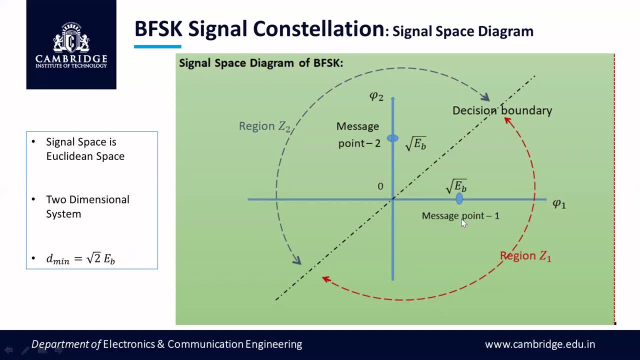 point 1 and symbol 1.. Similarly, second one is 0 root Ev. reverse Yes, This one. So 5-1 component is 0.. 5-2 component is root Ev. So these two points, what are? 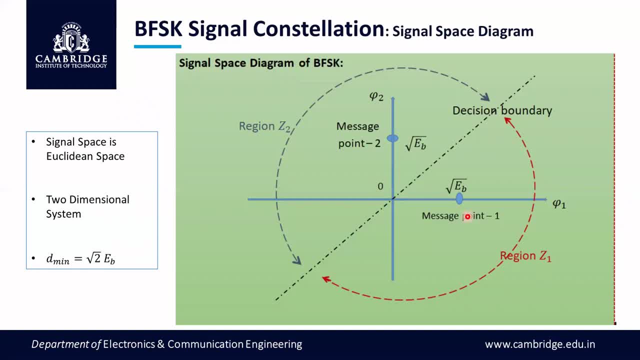 representing Two information signals. Right, So the two message points lie on two different axes. So two message points: First message point lie on 5-1 axis, Second one lie on 5-2 axis. So to establish decision. 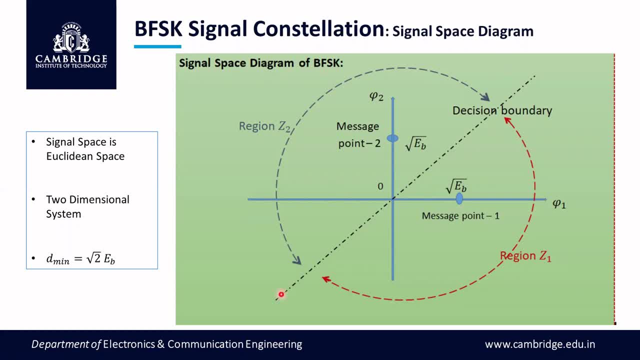 boundary. I have taken this dotted line. This will divide entire signal space into two equal parts. So this is taken as region 1 and this will taken as region 2.. In region 1, message point 1 falls. Region 2, message point. 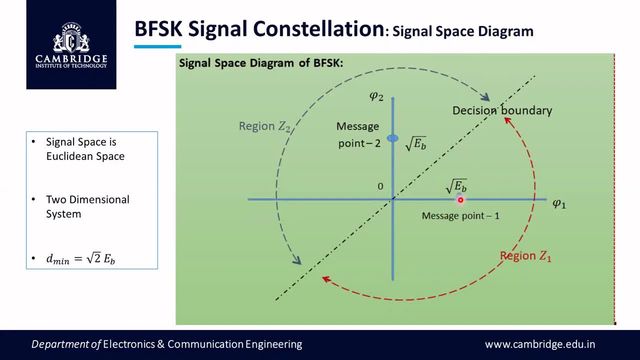 2 falls Right. So this is the voltage value with which signaling is transmitted for symbol 1.. But at the receiver, due to noise effect, this point may be shifted like this: this way: up to 0 point, So even. 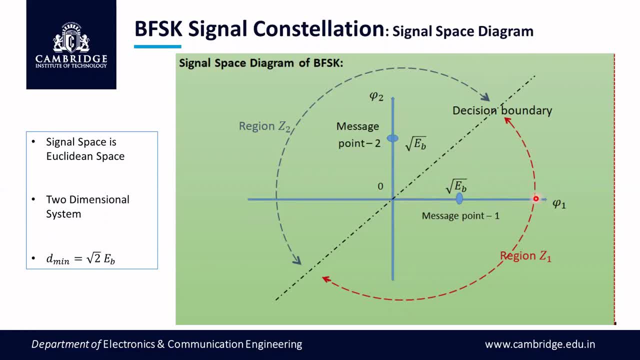 though it is shifting, changing due to noise anywhere on this axis, my decision still remains in favor of message point 1. Right. Similarly it is true for message point 2. But if this point shift this side of the boundary line, that is, 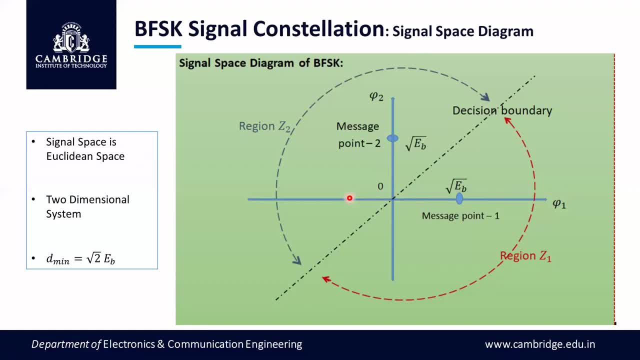 the other side of the boundary line. that time we may decide in favor of bit 0,, that is, symbol 0, that leads to error. Similarly, it is true for this message symbol also. So this boundary line is very useful. 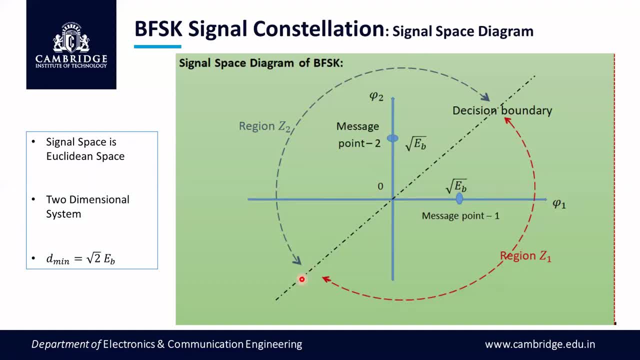 in deciding in favor of any of the symbols on the receiver. So this much gap is very important. Also, that is why I take this direct distance between these two. This distance is called this d minimum. This is going to be root 2 into eb. 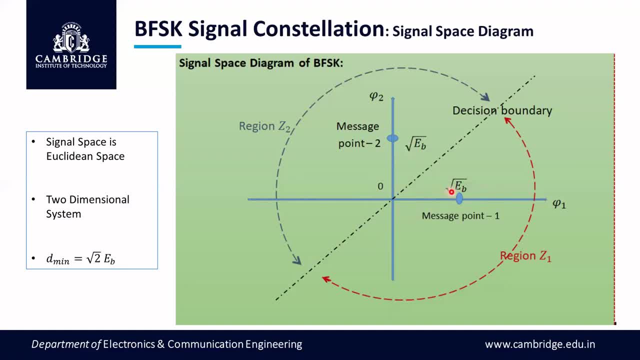 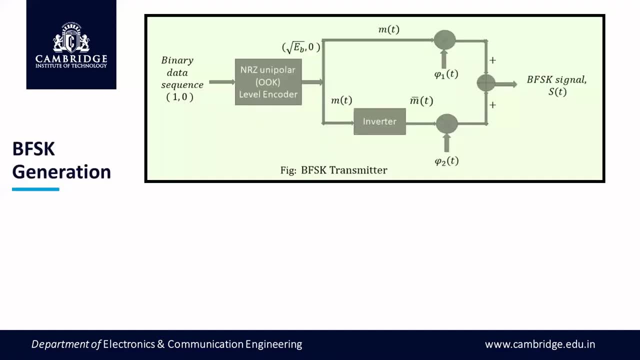 This is called d minimum, or Hamming distance according to light. Let us look into the generation of DFSK signal, that is, DFSK transmitter, based on the mathematical discussion made so far. Look at this one. This is binary information Which is converted to voltage values. 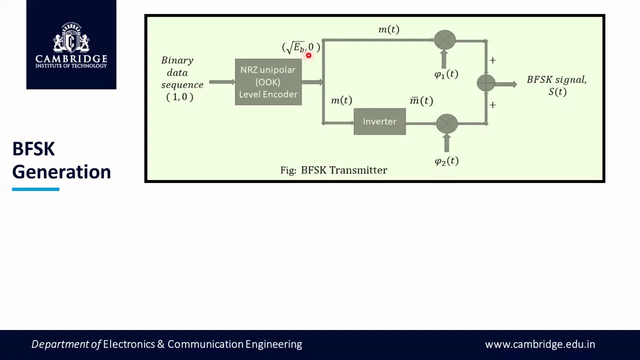 So 1 is converted to root eb and 0 is converted to 0. Using this level encoder- Since one of them is 0, it is called Arnoff Key technique, Unipolar signaling. Now the sequence 1 and 0. 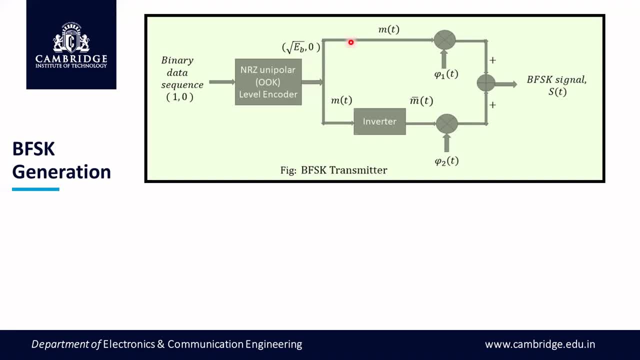 which are in the form of root, eb and 0, are given to two multipliers. These two multipliers are product modulators. That means they are multiplying to do the modulation. They are called modulators, But one of them is inverted and applied. 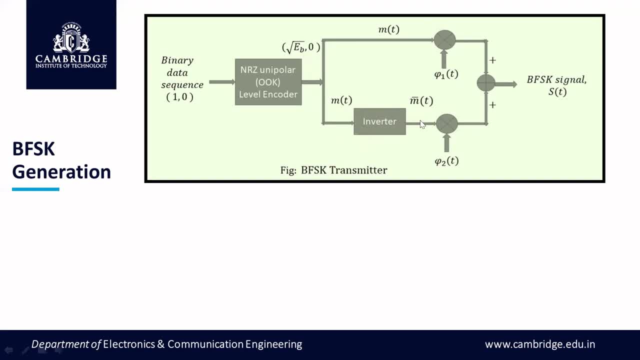 This m of t becomes m bar of t, Why? So let us see here. Look at this one. Assume that we are transmitting bit 1.. Bit 1 becomes the root eb. So root eb is the bit 1, let us say: 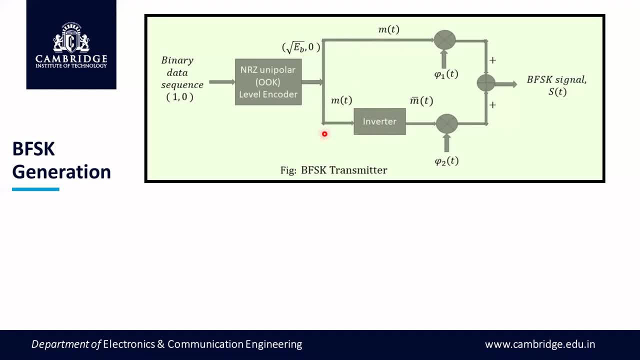 Bit 1 is applied here with the help of root eb. The bit 1 here, which is root eb, is inverted to 0.. So bit 1 is inverted to 0. like this inverter is designed, Designed inverter for that root eb. 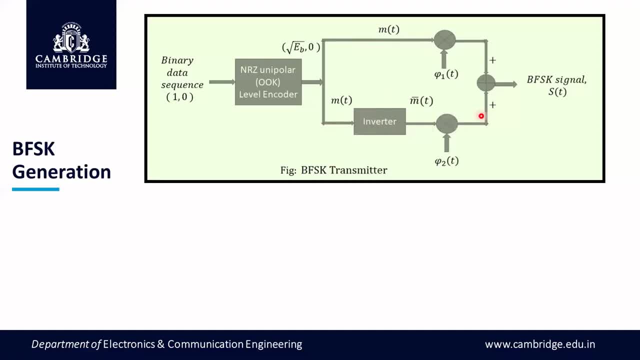 gets converted to 0 value And 0 value multipliers here will get 0 here. But here root eb into 5, 1 of t will come out here. So root eb into 5, 1 of t plus 0 will get root eb into 5, 1 of t. 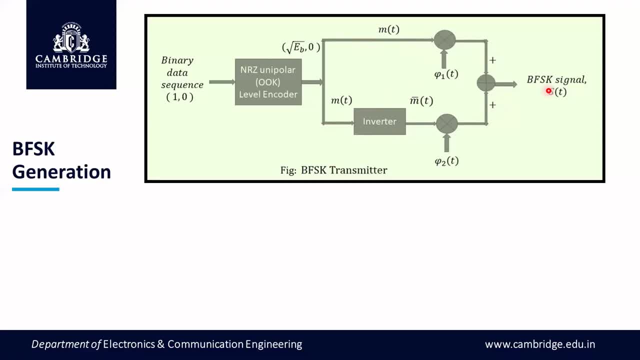 So root eb amplitude into 5. 1 of t represent your bit 1.. Even though there are two parallel multipliers or two parallel channels, still the output comes only from one channel. Other one will be in 0. The same thing happens in the other case also. 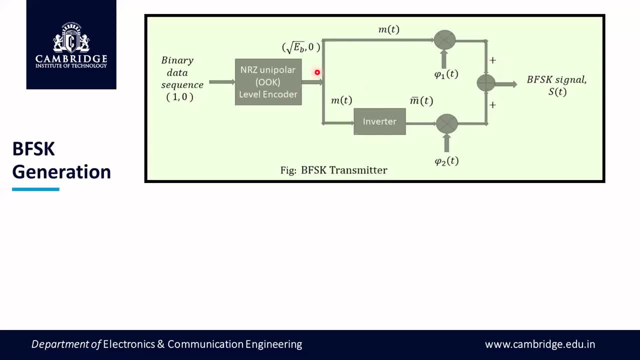 If you assume that this is 0, 0 represents here 0.. 0 applied to the upper channel, output is 0. But this 0, when given to inverter, it is converted to root eb. Root eb multiplies with 5, 1 of t. 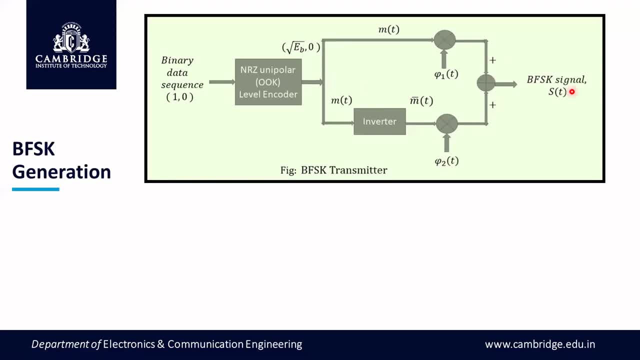 Here root eb into 5: 1 of t plus 0 is root eb into 5: 1 of t. That means at the output of the transmitter the signal is coming from only one of the channels, not both. One of them will be always 0.. 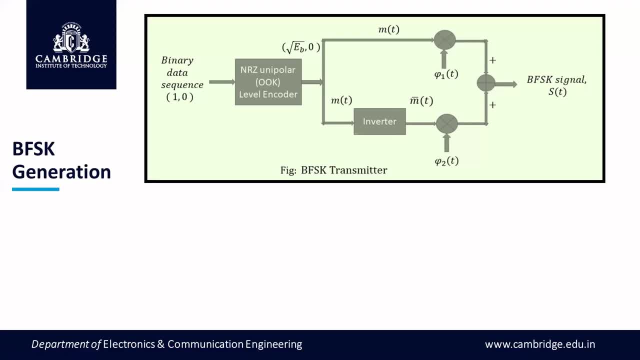 So if the signal is coming from the upper channel, the symbol transmitted is bit 1.. Coming from the lower channel, transmitted bit is 0.. The symbol 1 representation contains 5: 1 of t, Symbol 2, that is 0 bit. 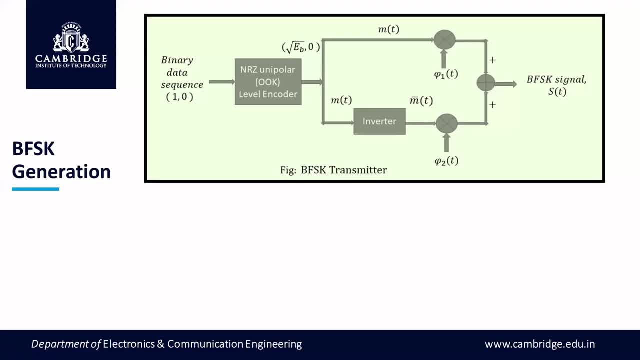 representation consists of 5, 2 of t. Keep this point in mind. Whatever I told so far is here. Same thing here: Level encoder and product modulators with 5- 1 and 5- 2.. Very important point to be noted here. 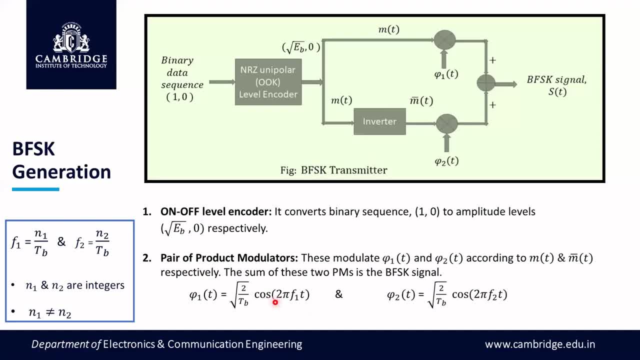 The frequency of form is N1 by Tb. Tb is one bit duration. In one bit duration of the input signal, our sine wave is in more cycles. You have seen in the waveforms already that in one bit duration there will be 3 cycles, 4 cycles. 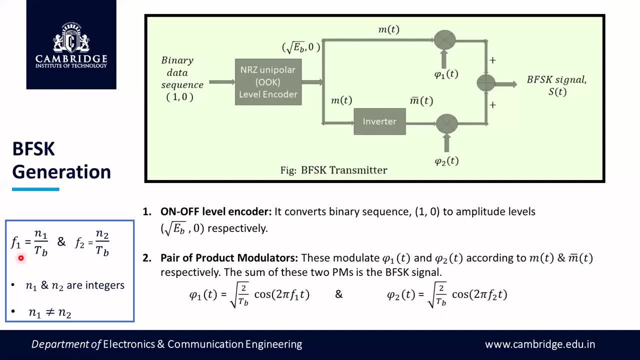 or 5 cycles like that In our calculating frequency. for example, if there are 5 cycles of sine wave in 1 Tb, this N1 is 5.. If there are 3 cycles of sine wave in 1 Tb, then it is 3.. 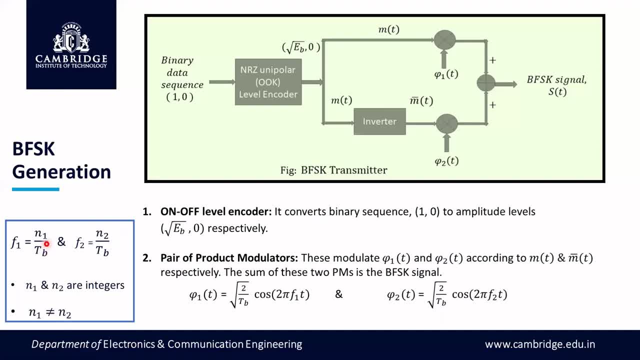 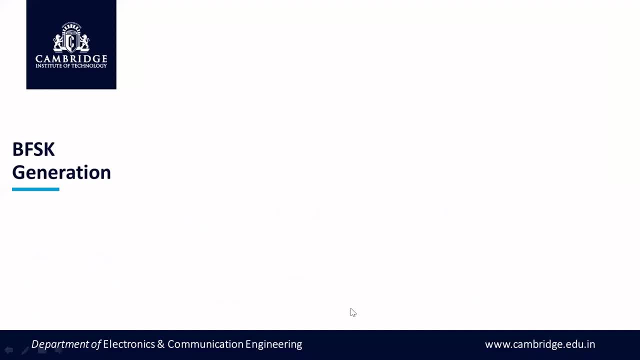 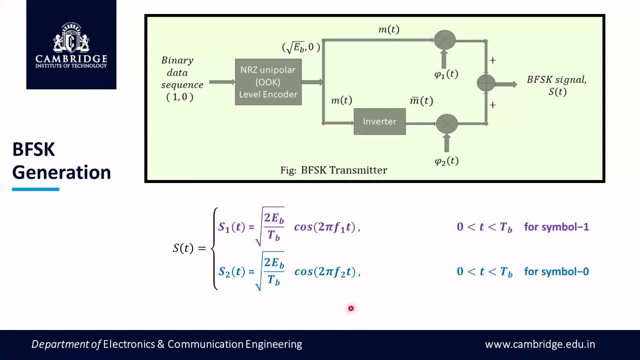 This. N1 and N2 are 2 integers, but not equal. They are going to tell you how many cycles of sinusoidal signal are present in 1 Tb. The same thing, what I have discussed earlier, is expressed in terms of 5: 1 and 5: 2.. 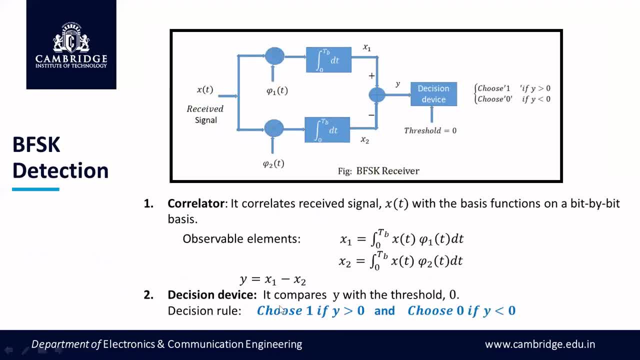 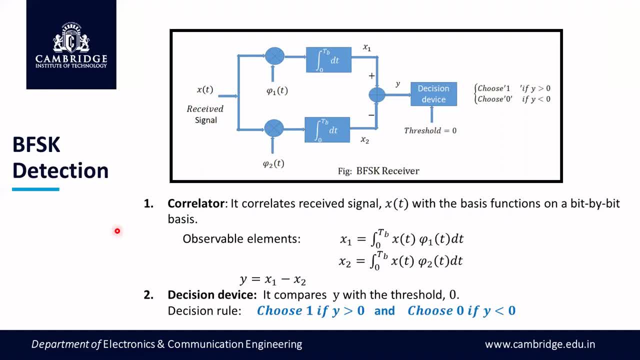 we are going to discuss about coherent detection. There are other techniques which involve non coherent technique also, which will be discussed later. So first let us know what is this VFSK- coherent detection. So take the received signal, multiply with 5, 1 after 1. 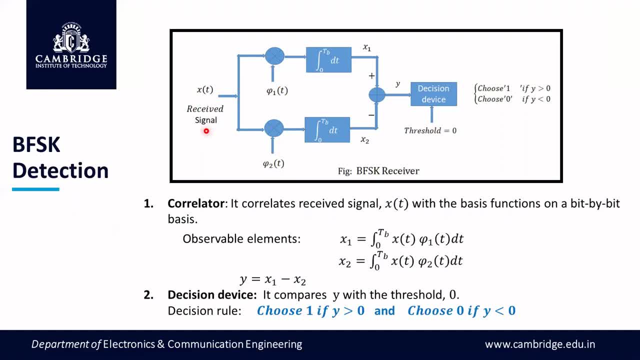 and 5- 2 after 1 parallel, Because at this point of time I don't know which symbol was sent: symbol 1 or symbol 0.. To check out which symbol was sent, I have to multiply with 5 1 and 5- 2 simultaneously. 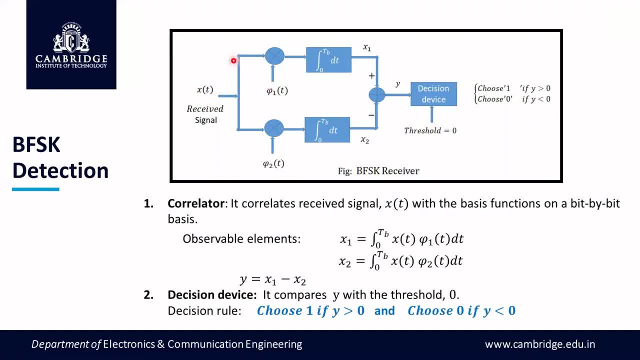 Because if the transmitted signal is bit 1, then it contains 5: 1, if the transmitted bit is 0, it contains 5, 2. So the corresponding multiplication will produce more output. So the corresponding multiplication will produce more output, Suppose the wrong basis functions are multiplied. 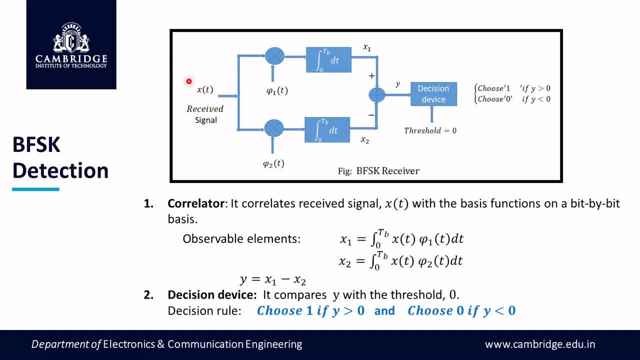 different basis functions are multiplied, they will produce 0. If the incoming signal is bit 1, which contains 5, 1 after t, then multiplying again with 5, 1 after t and integrating, as I said already, 5, 1 after t, already multiplied the transmitter. 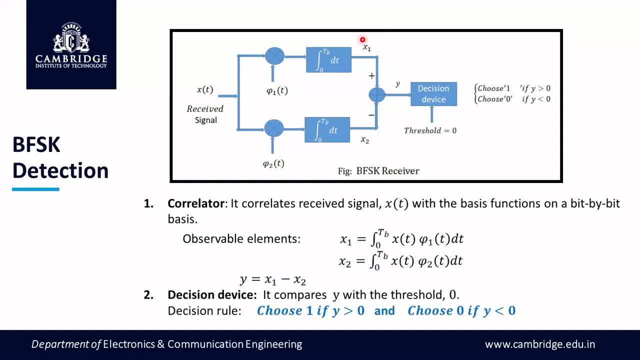 now we are multiplying the receiver and if you integrate we will get one value: x1.. But the 5 1 coming from input, when multiplied with 5 2, it will produce 0. It won't get absolute 0 here because there will be some noise component. 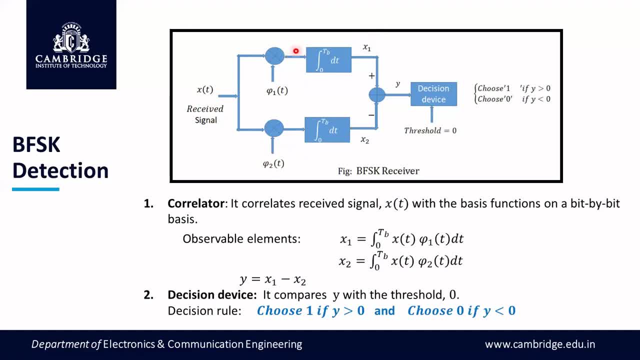 the noise component is here, is also there. so the signal component plus noise component is x1. Only noise component is x2.. Obviously x1 is more than x2.. So the positive value is more, negative value is less. So y value is the difference of these two. 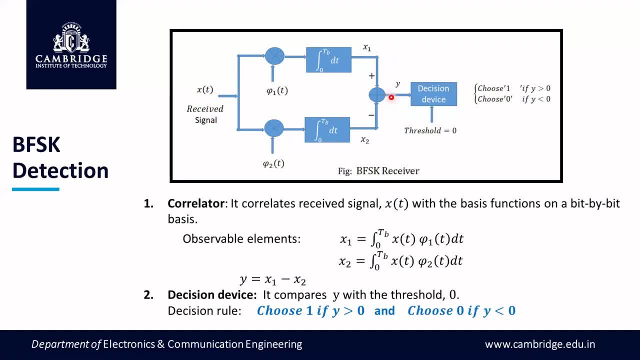 x1 minus x2.. So x1 is larger than x2.. That's why this y is positive and the y is positive greater than 0. we choose in prayer. We decide in favor of 1.. Similarly, if it is 0, the symbol 0 is transmitted. 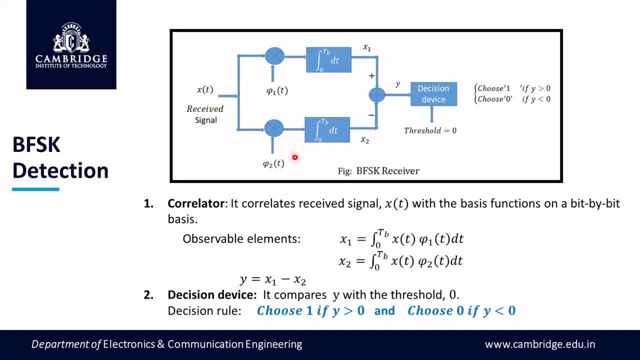 What happens that time? The transmitted signal contains 5, 2 after t. So 5, 2, 5, 2. multiplication and integration gives one good value of x2, and this goes to 0. 5 1 and 5: 2. 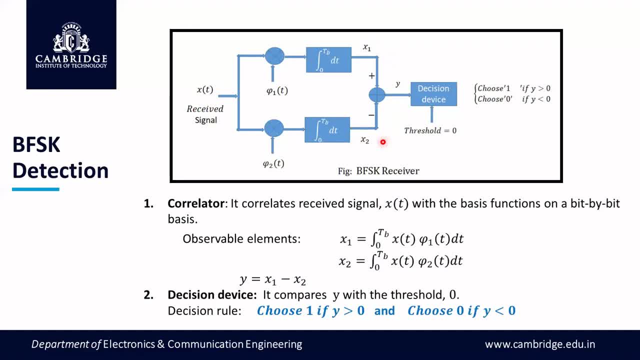 multiplication and integration goes to 0. So x1 is smaller, x2 is larger, Positive value is smaller, Negative value is larger, y is negative. So this is how this works. That's why the threshold is taken as 0, because 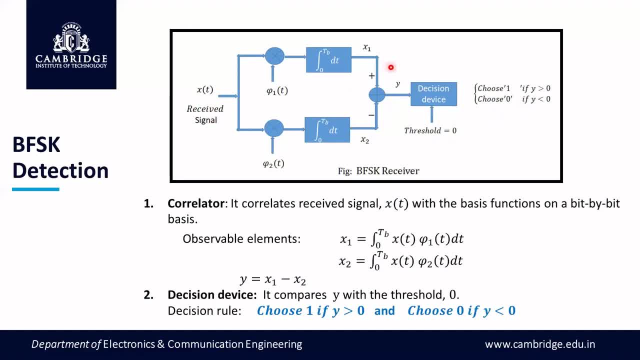 one will be positive, y will be positive, sometimes negative, sometimes, depending on the symbol. So I guess you have understood of this one. Whatever, the operation explained here is given in the form of equations. here x1 is multiplication of x of t and 5 1 of t and integration.